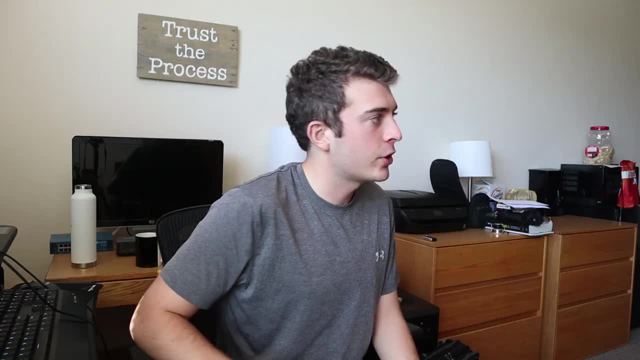 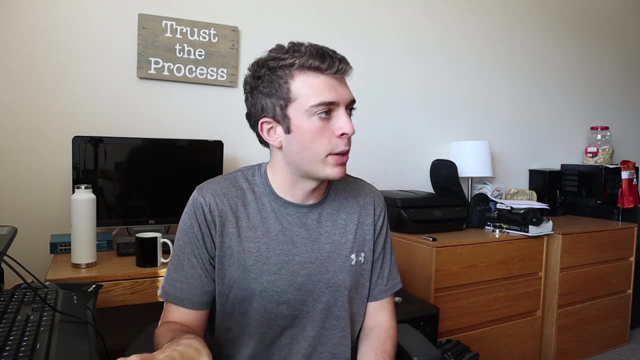 Oh, that's a violation of the compliance standards. I'm sorry I didn't. I didn't mean I didn't know that we had to be in compliance with physical security operations. I'll clean this up, I promise. According to my violations here, you are going to have to be reported to your upper level. 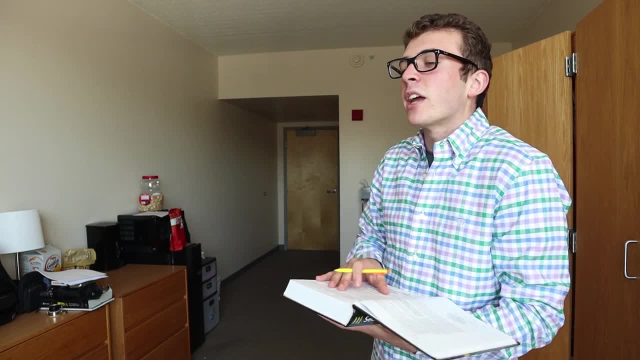 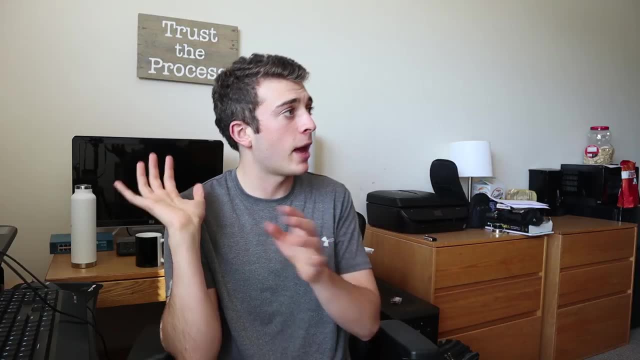 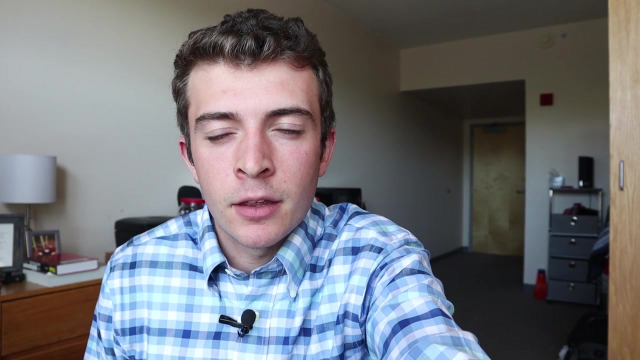 supervisor and you are in breach and not compliant with any of physical security operations. meaning No, no, no, no, you don't need to report to my advisor. I promise I won't. I just need to just clean up some things. Have a good day, sir. Now that was some good class A acting right there. 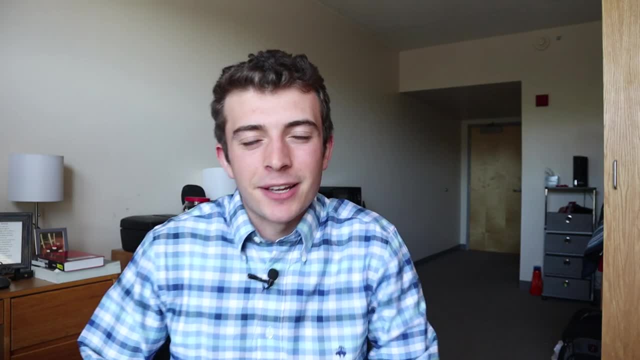 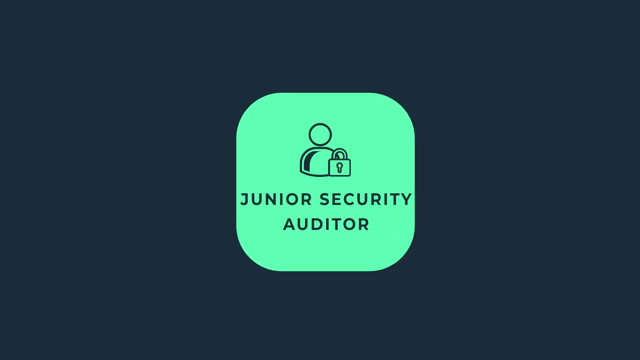 Hey, what's up, guys? Grant Collins here, And today I'm going to be talking about junior security auditor and what the junior security auditor does in cybersecurity. So, without further ado, let's go ahead and get started. A junior security auditor is going to. 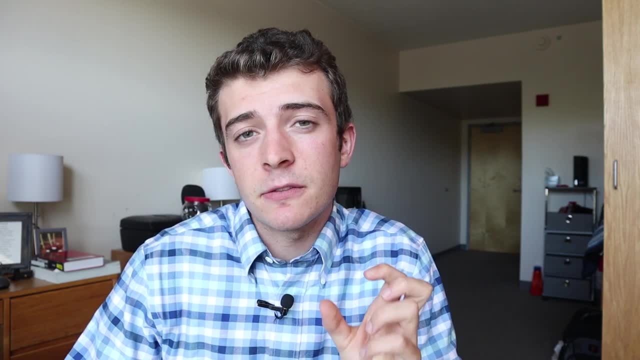 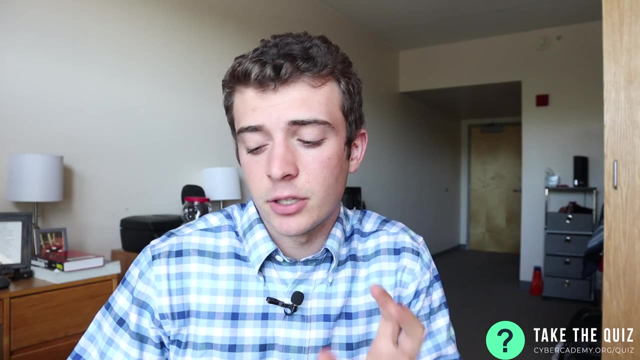 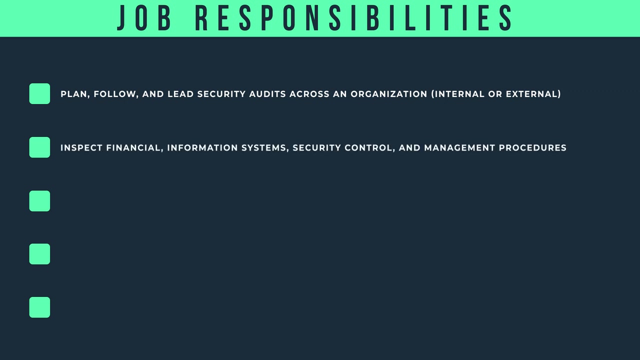 perform a thorough analysis of the safety and effectiveness of computer systems and their related security components within an organization. These include planning and following and leading security audits across an organization- internal and external. inspect financial information systems, security controls and management procedures. evaluate the efficiency effectiveness. 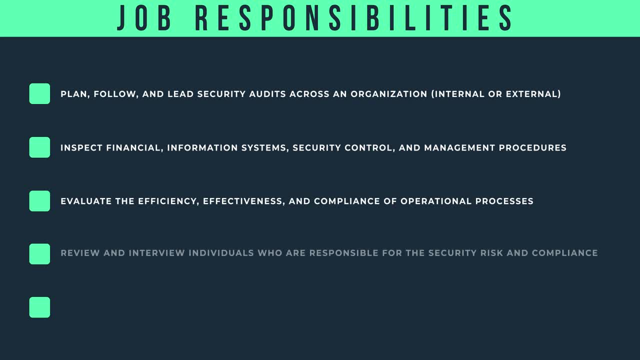 and compliance of operational processes. review and interview individuals who are responsible for the security, risk and compliance properly. document audit process among a variety of computing environments and computer applications. access potential exposures and failures. evaluate the relevancy, accuracy and perspective of audit e-mails. and evaluate the effectiveness and compliance of operational processes. 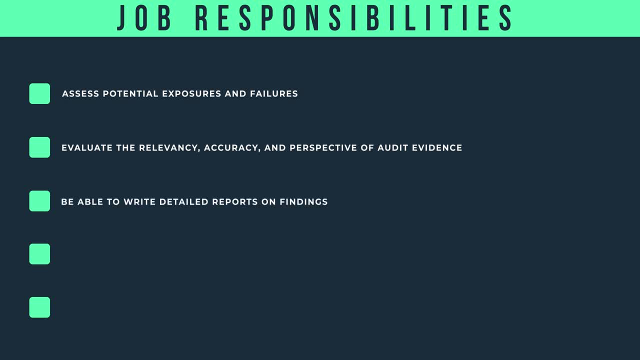 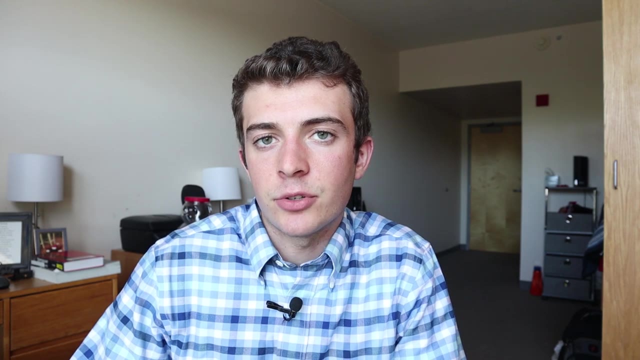 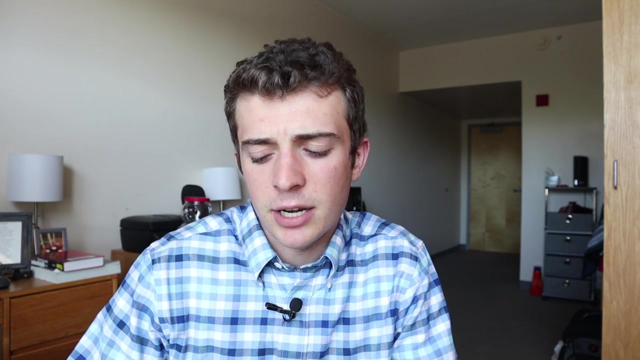 A junior security auditor is going to do a wide array of things And oftentimes they're going to go into organizations and basically assess their overall security posture and then give best practices Now, because you are a security auditor and you're going to be traveling a lot. your salary ranges, but the basic or the general average for a junior security auditor is between $50,000 and $105,000 per year in the United States. Regarding past work experience, usually you have to have around three to six years before you can get into this position. In terms of degree,